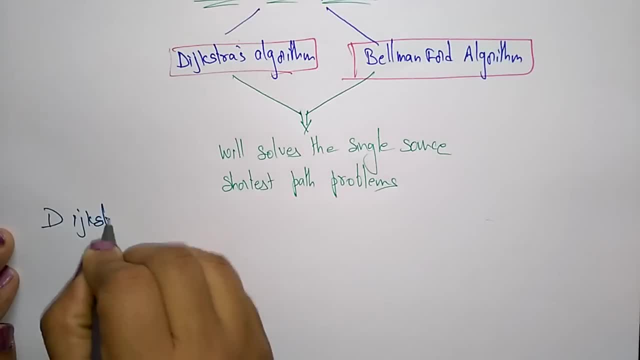 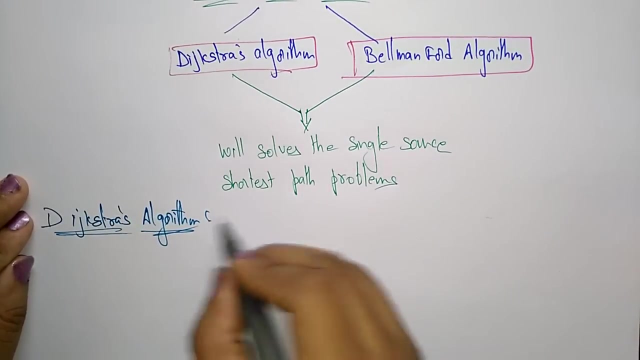 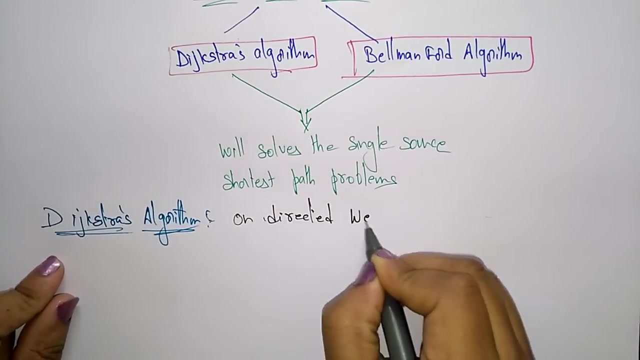 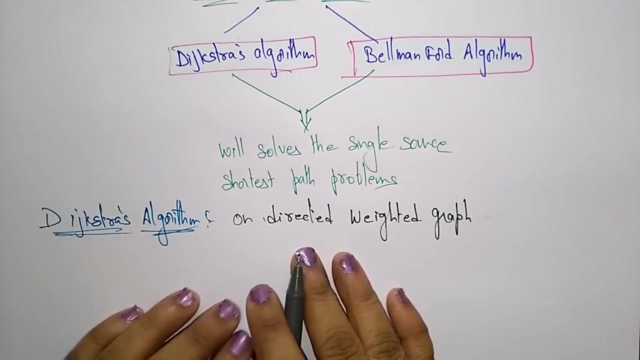 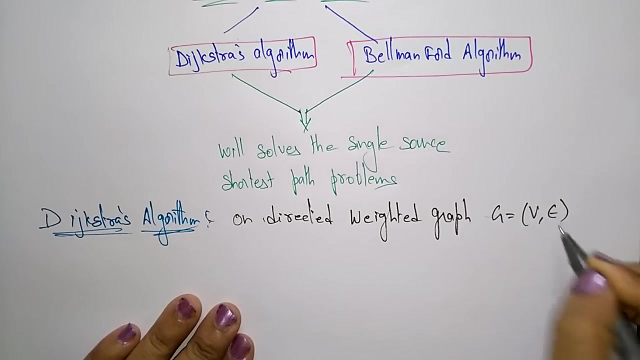 Dijikstra's algorithm. So this Dijikstra algorithm solves the single source shortest path problems on a directed. So this is based completely on directed weighted graph. So the one thing you have to be noted- that Dijikstra algorithm is completely based on the directed Directions- will be there A directed weighted graph of G consisting of vertices and edges. 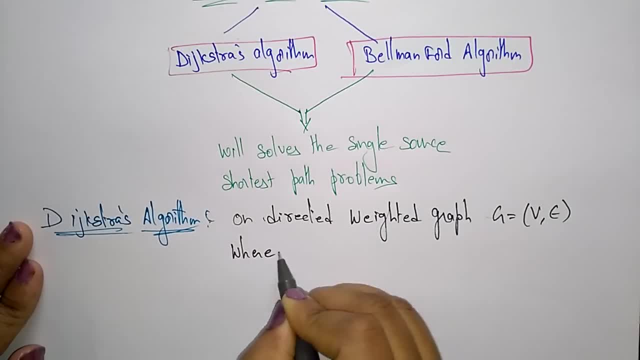 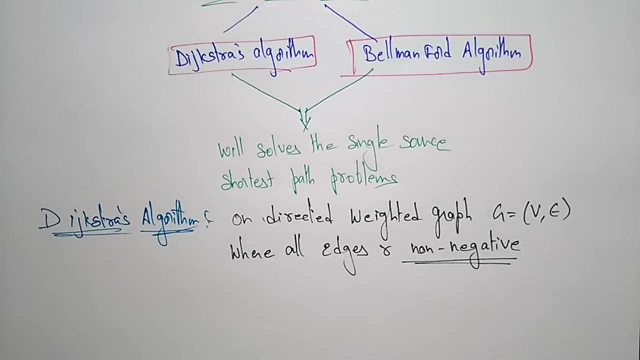 So where all edges are non-negative. So whatever the edges that are present in Dijikstra algorithm, that should be non-negative, Whereas in Bellman-Ford algorithm you can include the negative edges also. But the difference between these two is Dijikstra algorithm have the edges which are non-negative numbers. 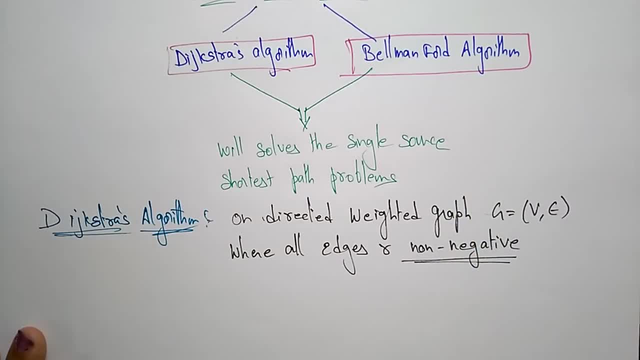 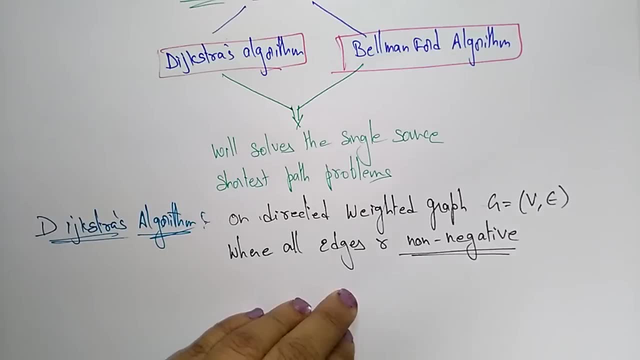 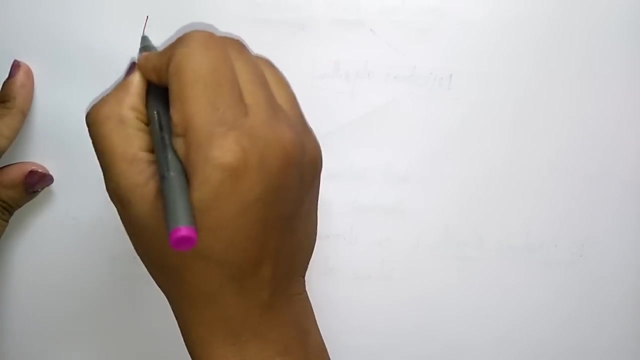 Whereas Bellman-Ford algorithm can access, But the negative number edges also. Now let us see this algorithm of Dijikstra algorithm. What is the algorithm? Let me write the algorithm of this method, Dijikstra's algorithm. 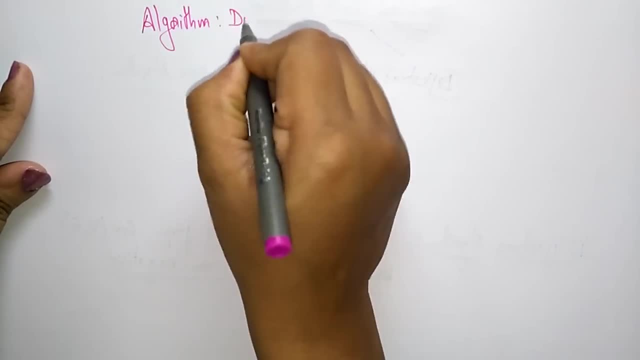 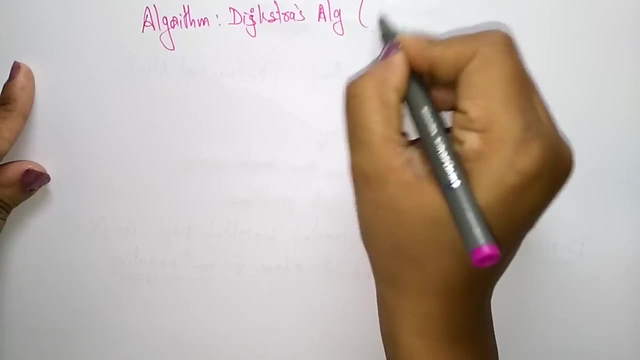 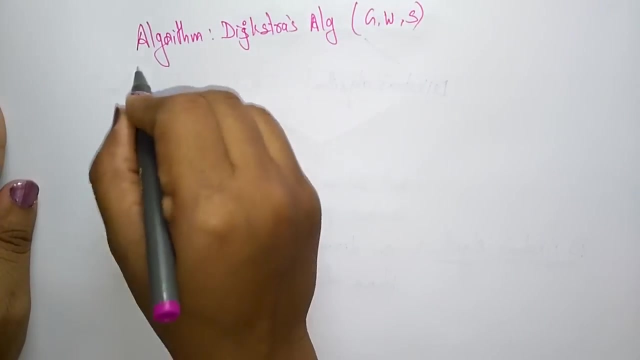 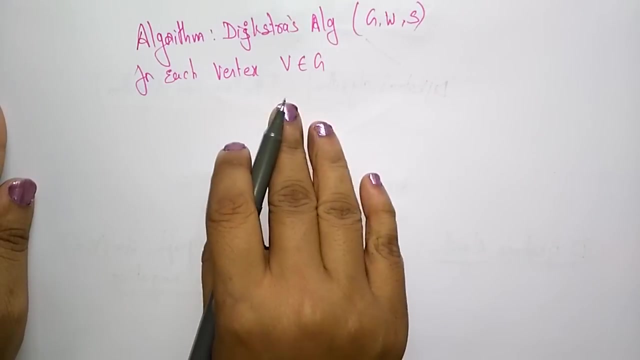 Dijikstra's algorithm. G is the graph, W is the weight of that edge And S is the set For each vertex. vertex belongs to the graph, So that vertex should present in the graph. So V, dot D. 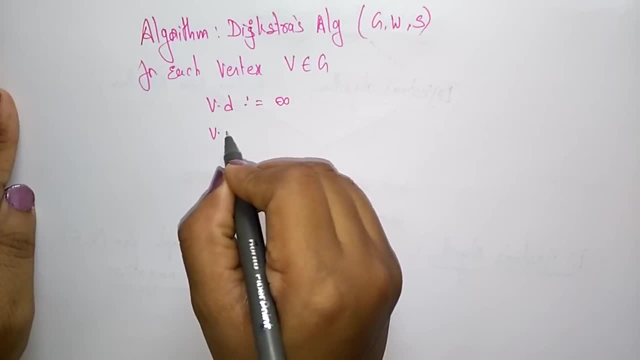 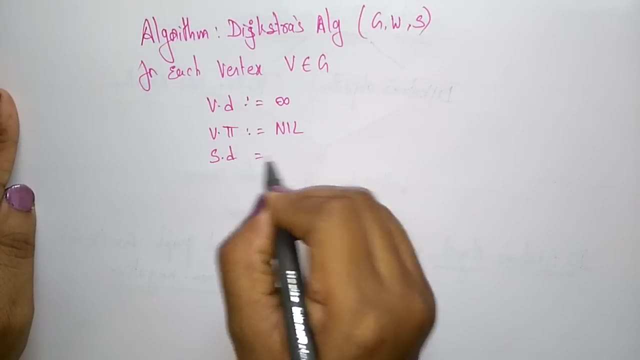 For starting. it should be initialized to infinity, It should be nil And S dot, D, distance should be zero And the starting edge should be indicated phi And the Q. whatever the Q, that should be G graph dot vertex. So here the condition. 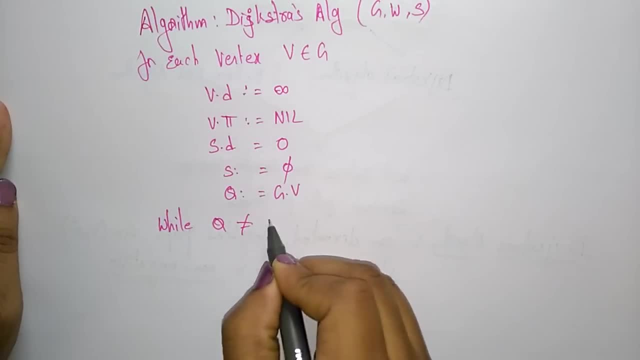 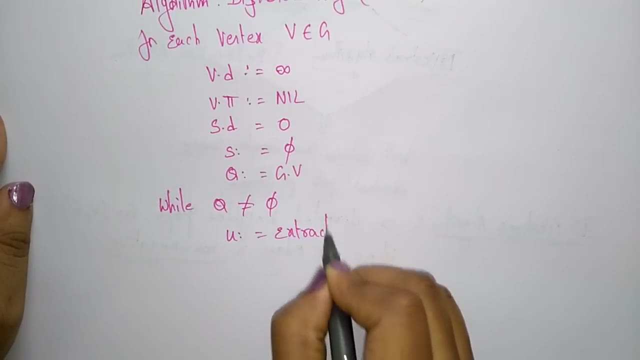 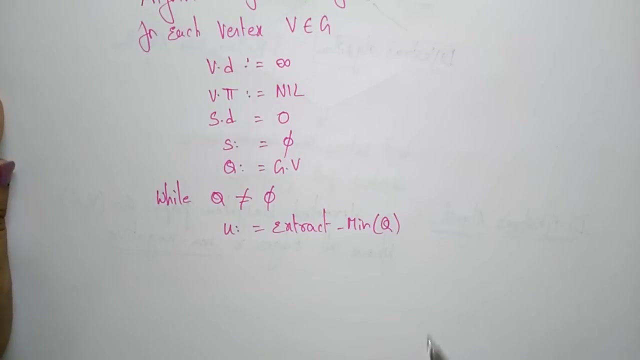 First, simply, I am writing the algorithm Afterwards. I will take the example How we will solve the Dijikstra algorithm To find out the shortest path: Extract, Extract min of Q means the extract min is a function which is select the extract, the minimum edge. 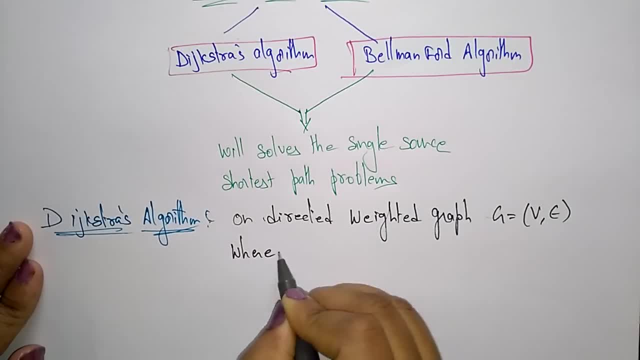 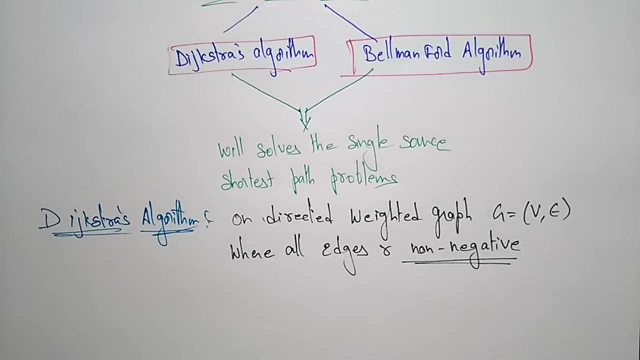 So where all edges are non-negative. So whatever the edges that are present in Dijikstra algorithm, that should be non-negative, Whereas in Bellman-Ford algorithm you can include the negative edges also. But the difference between these two is Dijikstra algorithm have the edges which are non-negative numbers. 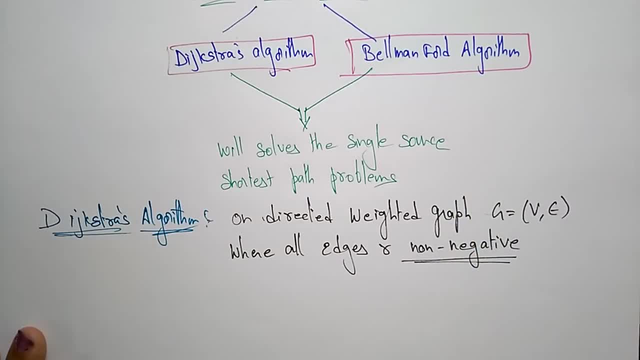 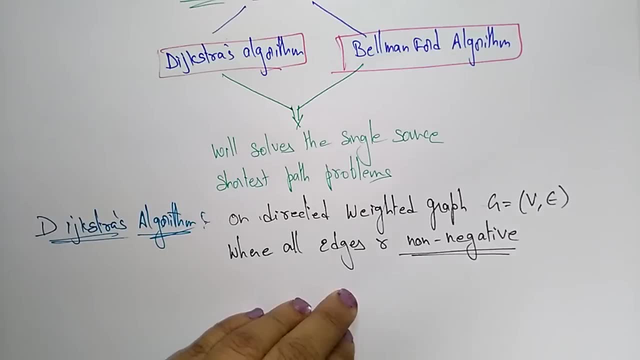 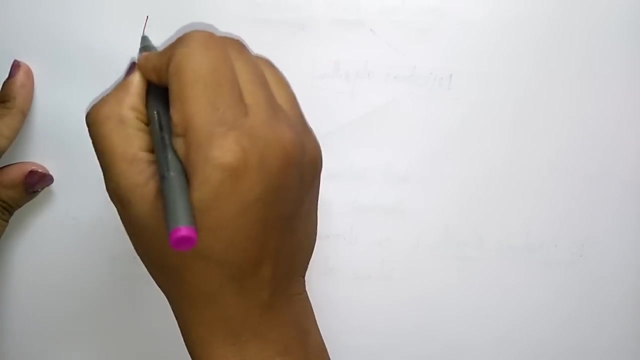 Whereas Bellman-Ford algorithm can access, But the negative number edges also. Now let us see this algorithm of Dijikstra algorithm. What is the algorithm? Let me write the algorithm of this method, Dijikstra's algorithm. 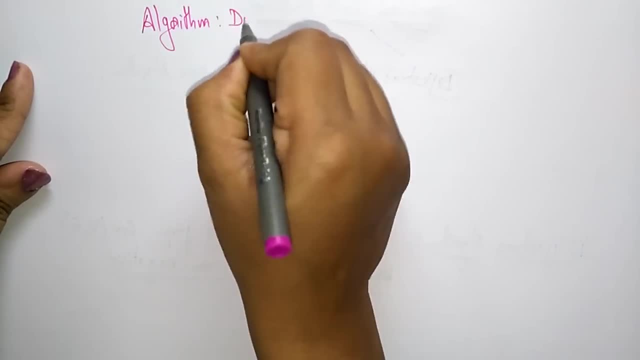 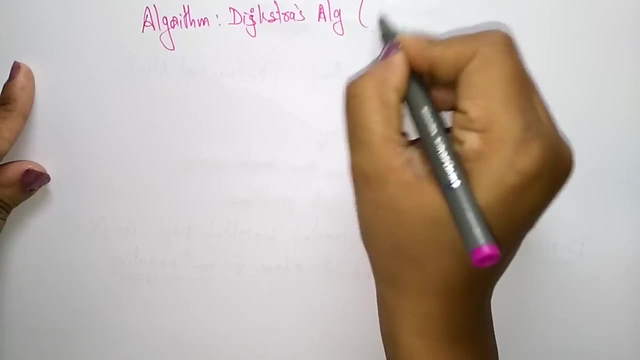 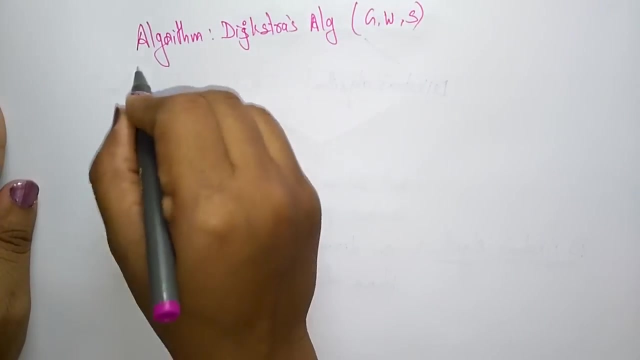 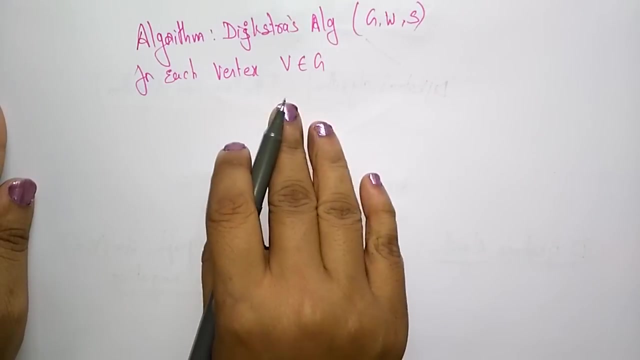 Dijikstra's algorithm. G is the graph, W is the weight of that edge And S is the set For each vertex. vertex belongs to the graph, So that vertex should present in the graph. So V, dot D. 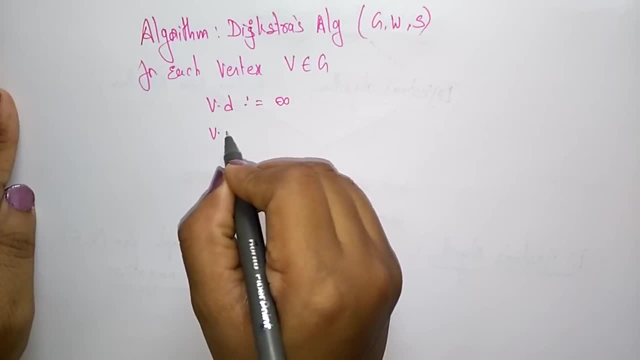 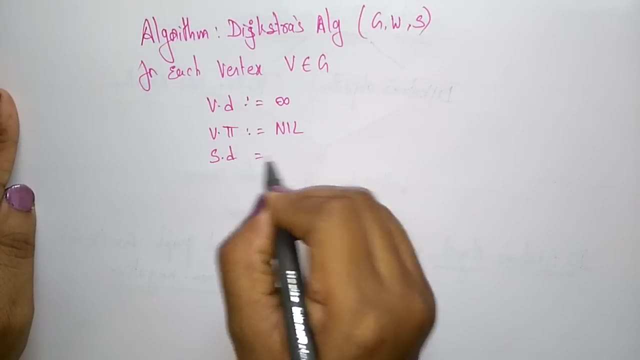 For starting. it should be initialized to infinity, It should be nil And S dot, D, distance should be zero And the starting edge should be indicated phi And the Q. whatever the Q, that should be G graph dot vertex. So here the condition. 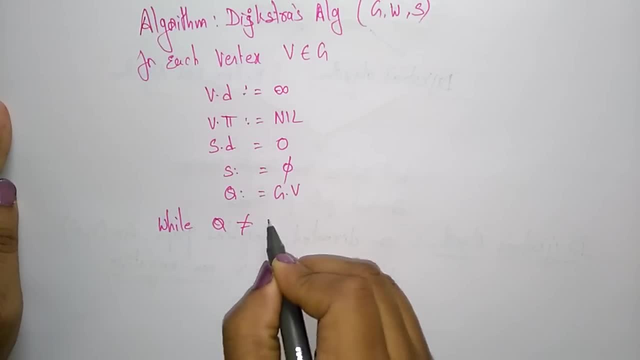 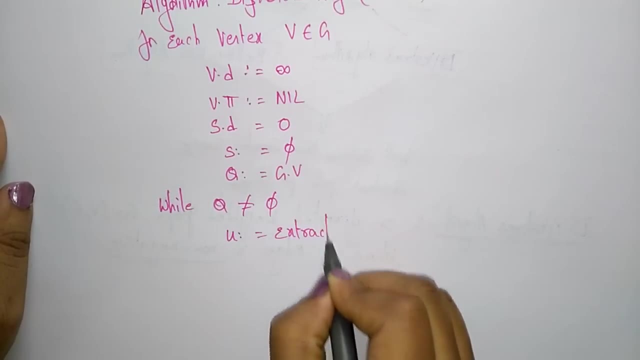 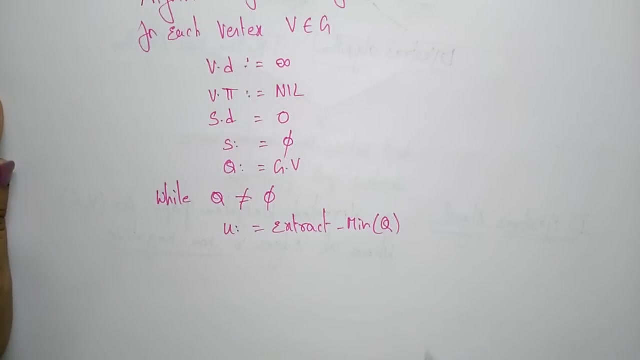 First, simply, I am writing the algorithm Afterwards. I will take the example How we will solve the Dijikstra algorithm To find out the shortest path: Extract, Extract min of Q means the extract min is a function which is select the extract, the minimum edge. 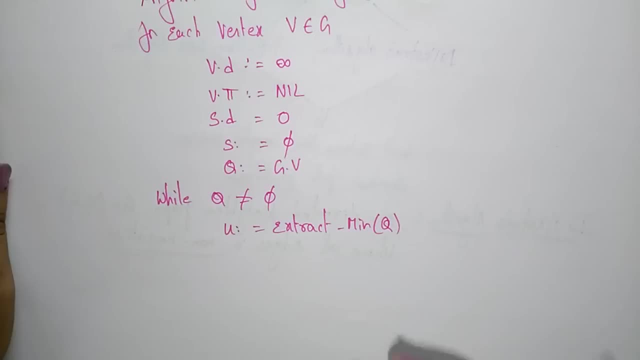 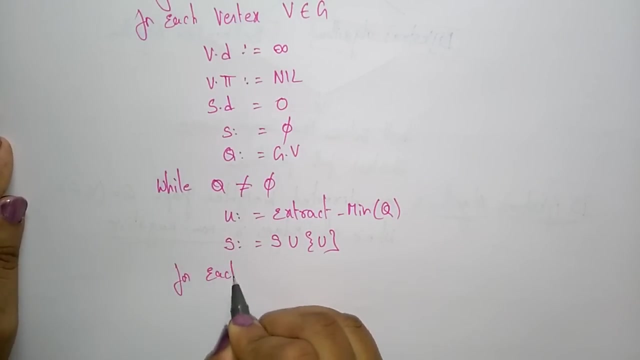 That is present in the graph. That acts as a key. That acts as a sample key. Extract min S is equal to union of. You have to combine that extract minimum value with the set For each vertex. V belongs to G dot edges of U. 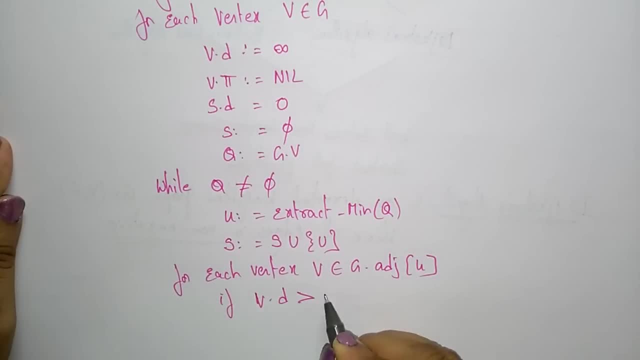 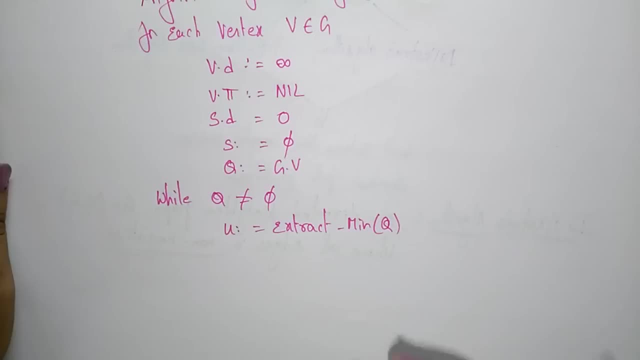 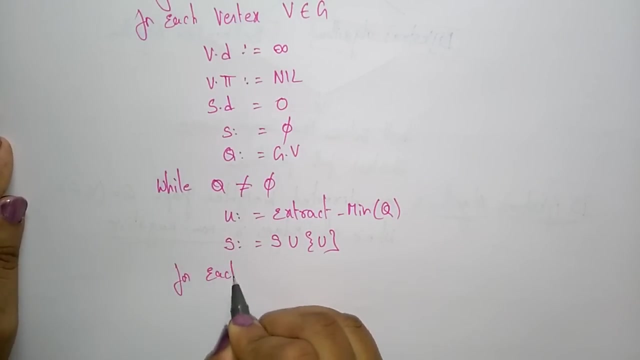 That is present in the graph. that acts as a key. That acts as a sample key. Extract min S is equal to union of. You have to combine that extract minimum value with the set For each vertex. V belongs to G dot edges of U. 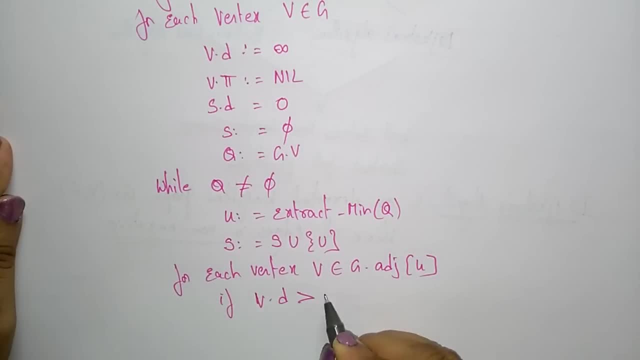 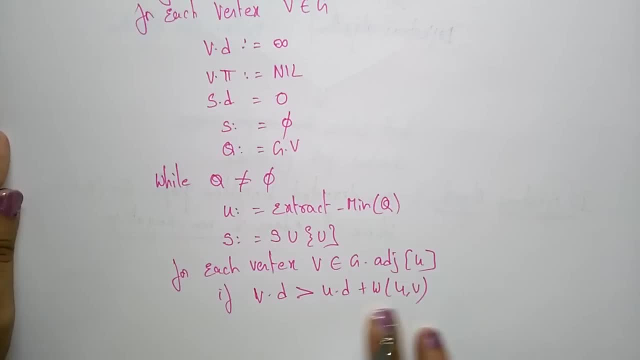 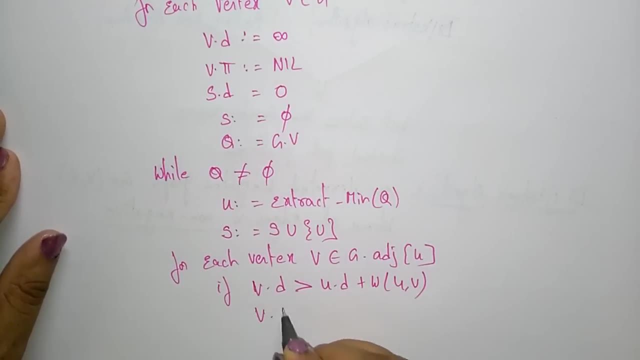 So this is the set, So these are the edges. Okay, For that vertex and that should be. If this weight should be greater than the vertex, dot D, Then you have to take V dot D is equal to U dot D plus W of U comma V. 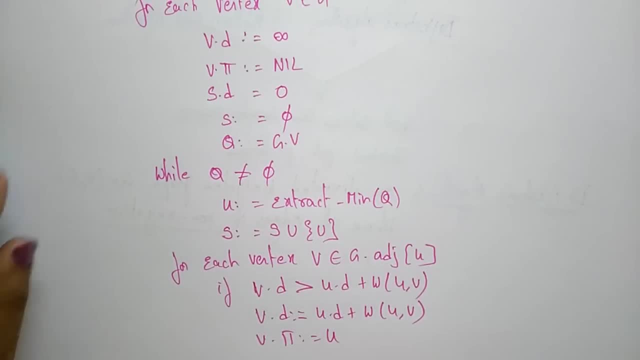 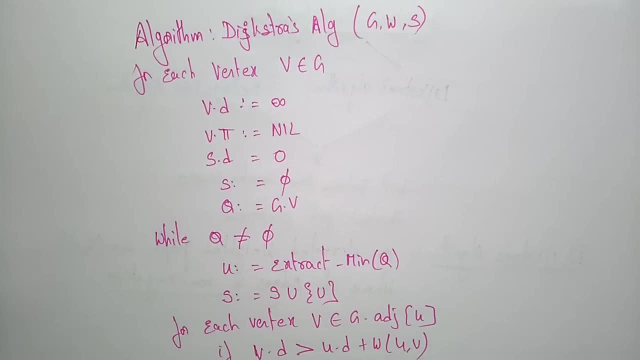 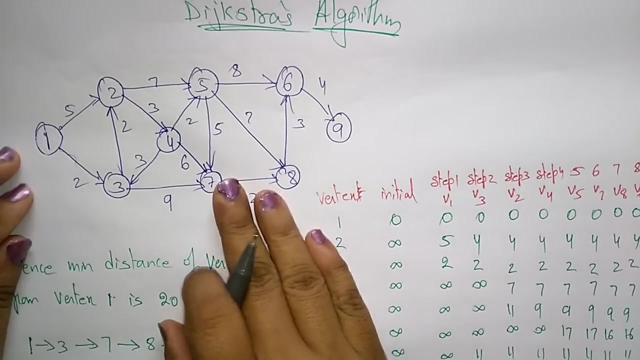 And finally you make V dot. pi is equal to U. So this is the algorithm for the Dijikstra method. Now let us take the example. So here, this is an example, this is a graph. so let us consider the vertex 1 and the 9 we have to reach from vertex 9 to. 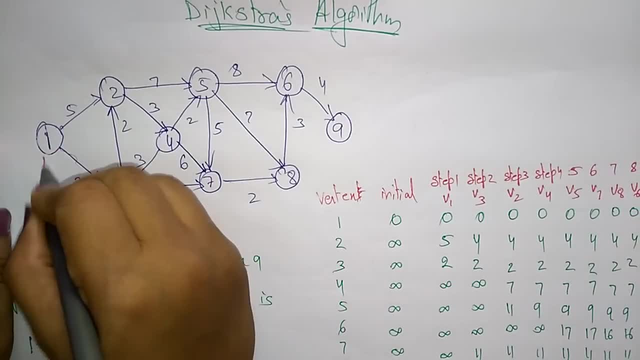 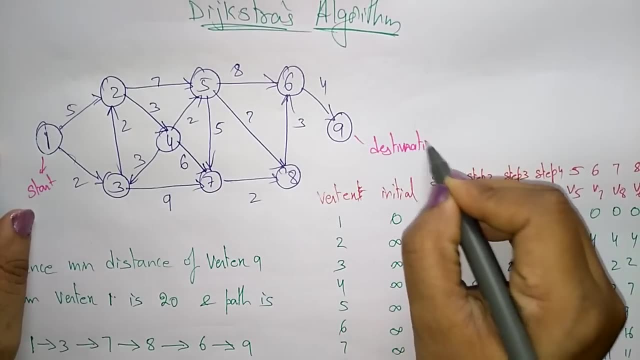 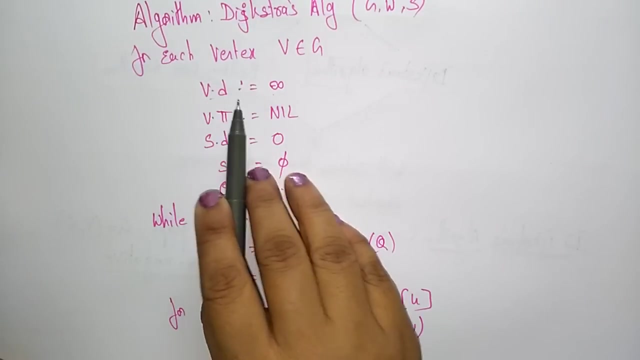 1 to 9. as a start. this is a start, this is a start and this is the destination. so in the previous algorithm i said s is for the start, the set s is start and d it should be destination. the vertex of the destination should be: make it as infinity. okay, and the starting. 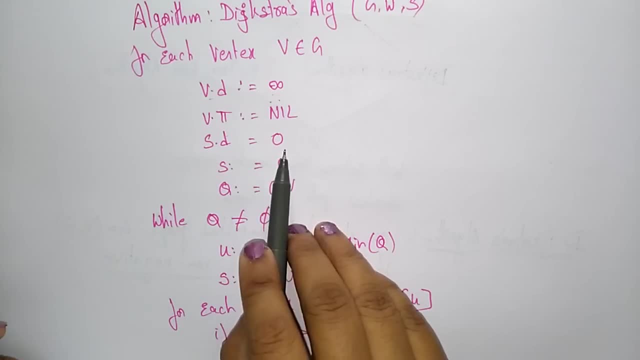 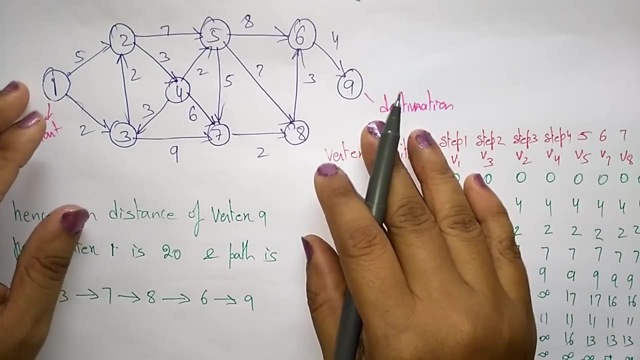 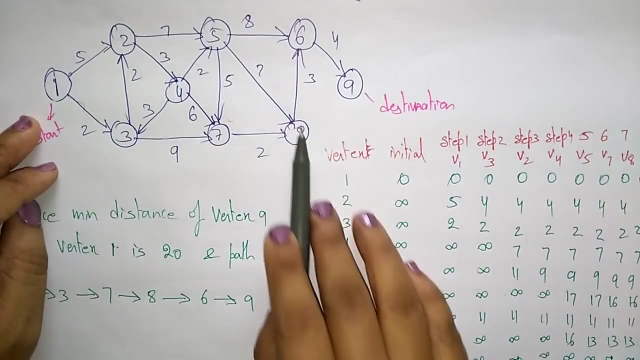 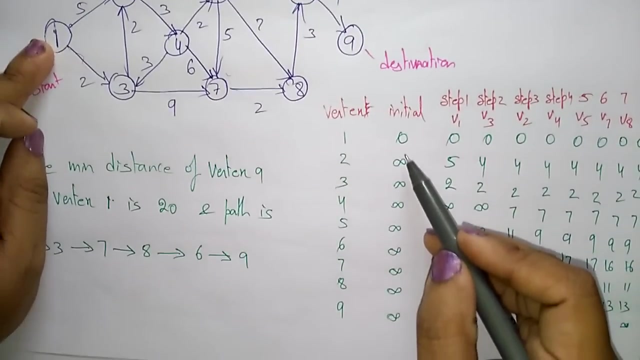 vertex, the start dot d should start with the zero. okay, so this is the start and this is the destination here. so the vertex, destination, vertex, respectively, initially all vertices. so whatever the vertices is there, initially, all vertices except the start vertex are marked as infinity. so here i marked, except the start vertex. so this is a start vertex, except the start vertex i make. 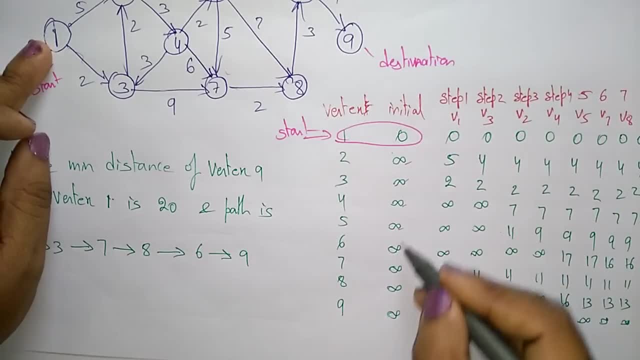 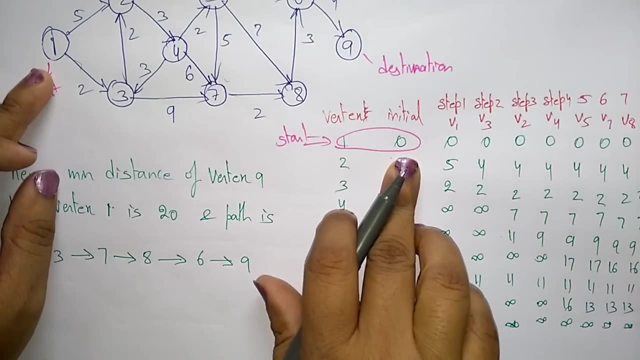 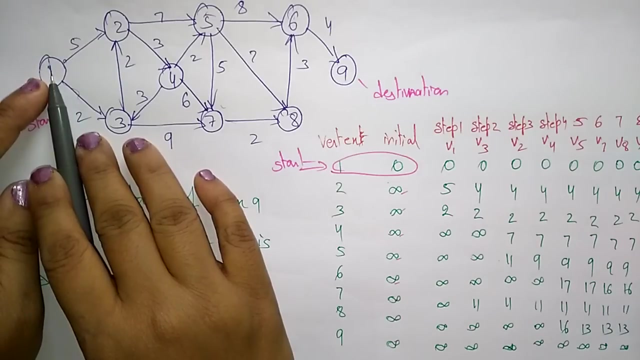 all the vertex or infinity, mark it as infinity. so next, uh, and the start vertex is marked as zero. so now we have to be checked for vertex. we uh from starting from the vertex v1. so the edge we have to take: the five, the, the it reached to the two. okay, 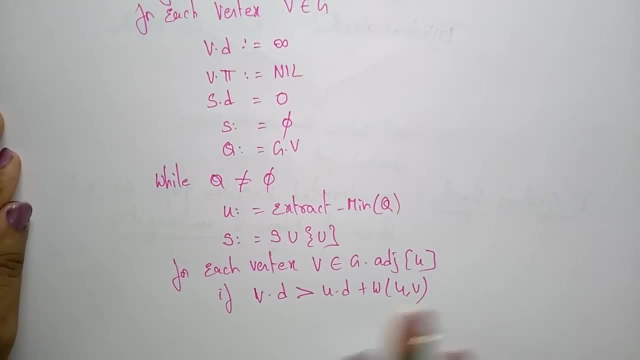 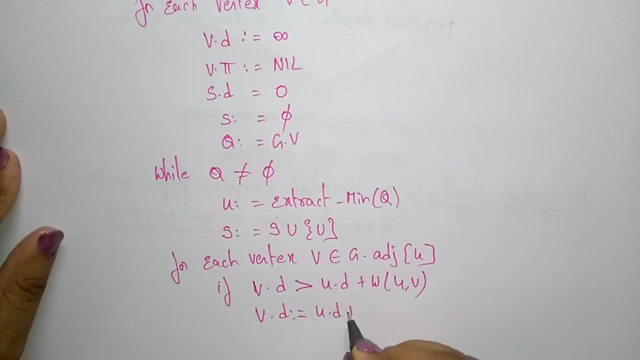 Okay, for that vertex, And that should be, this weight should be greater than the vertex, dot D. Then you have to take V dot D is equal to U dot D plus W of U comma V And finally you make V dot pi is equal to U. 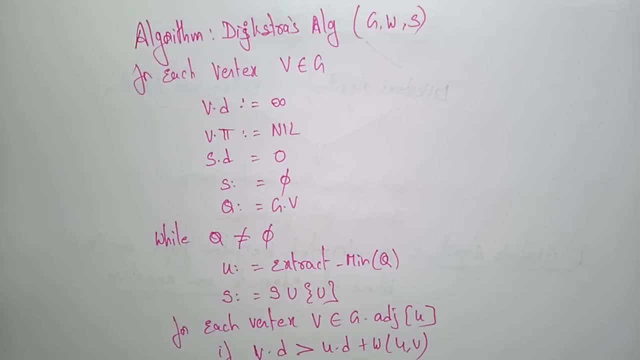 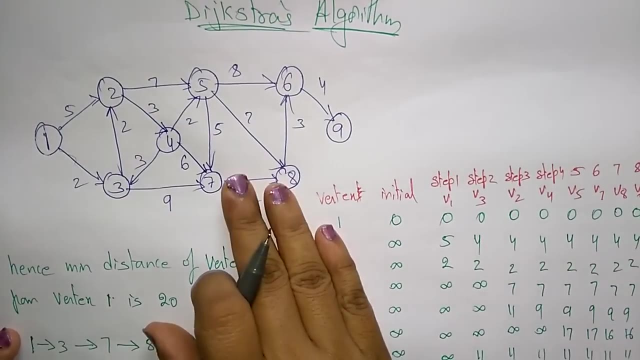 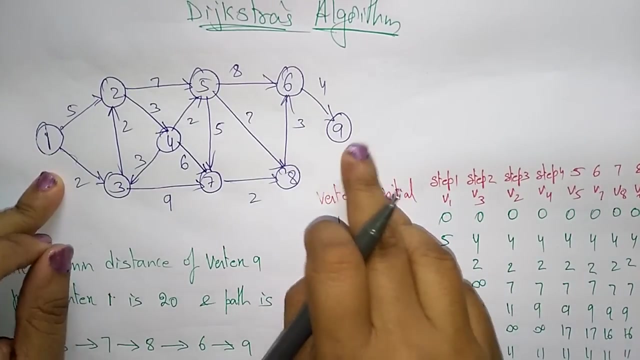 So this is the algorithm for the Dijikstra method. Now let us take the example. So here this is an example, This is a graph. So let us consider the vertex 1 and the 9. We have to reach from vertex 9 to 1 to 9.. 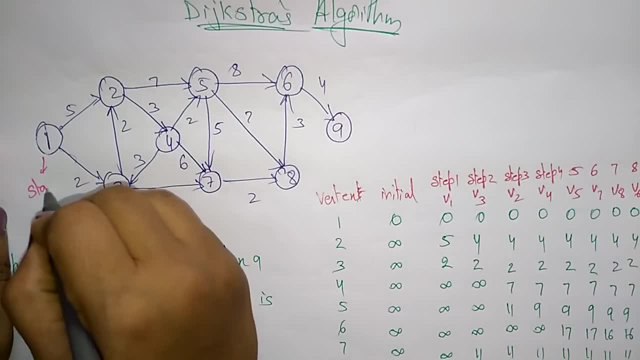 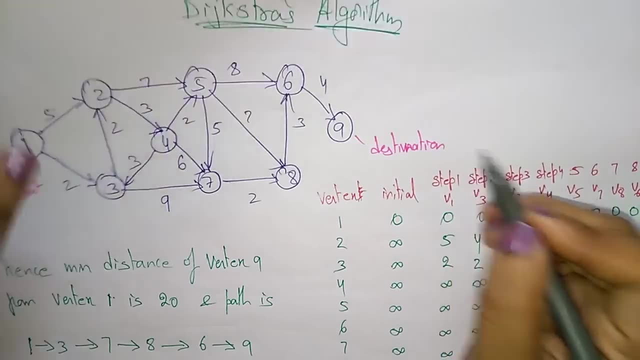 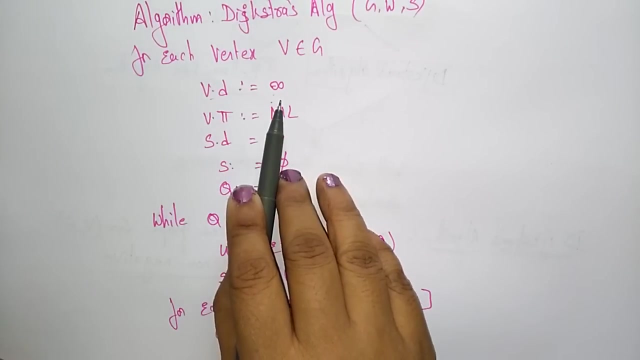 As a start. this is a start. This is a start and this is a destination. So in the previous algorithm I said S is for the start, the set S is start and D it should be destination. The vertex of the destination should be: make it as infinity. 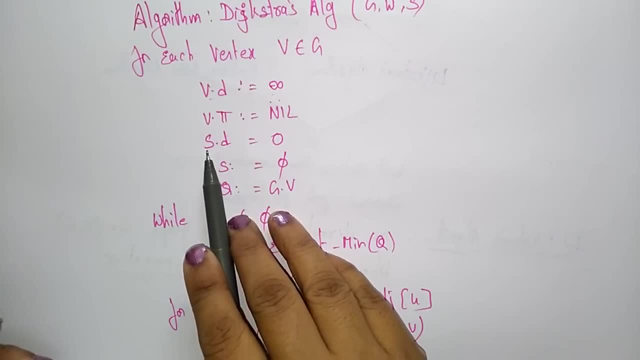 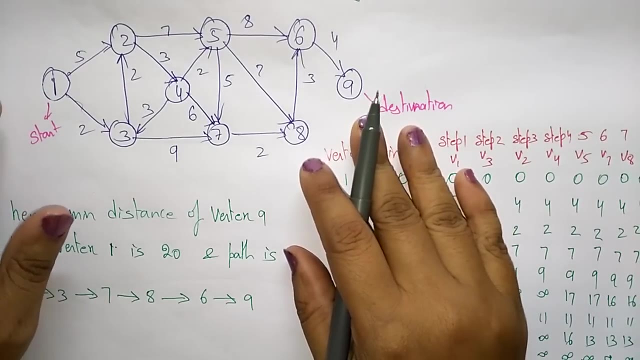 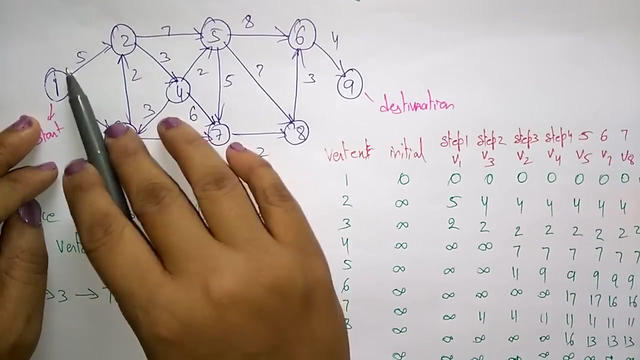 Okay, and the starting vertex, the start dot D, should start with the 0.. Okay, so this is a start and this is the destination here. So the vertex, destination, vertex, respectively, Initially all vertices. so whatever the vertices is there. 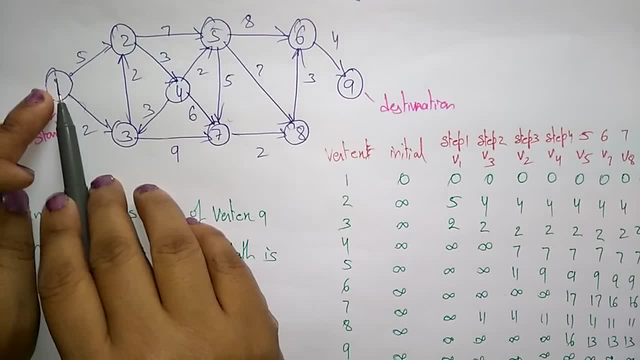 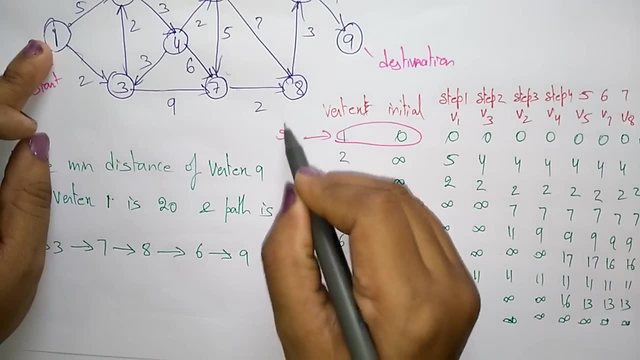 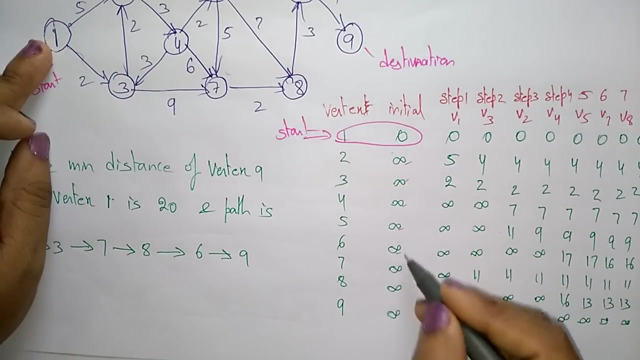 initially all vertices except the start vertex are marked as infinity. So here I marked except the start vertex. So this is a start. Except the start vertex I make all the vertex are infinity. Mark it as infinity. So next, 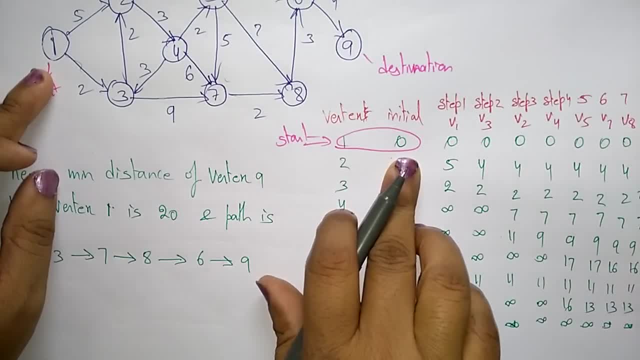 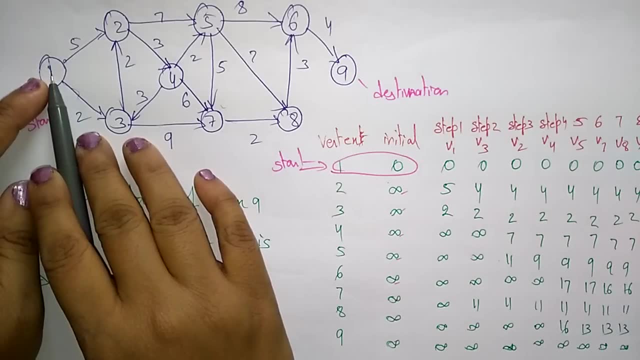 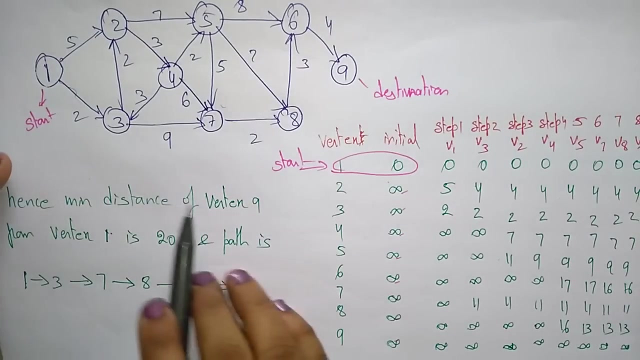 And the start vertex is marked as 0. So now we have to be checked for vertex from starting from the vertex V1.. So the edge we have to take, the 5, it reaches to the 2.. Okay, so here we have to find the minimum distance of vertex. 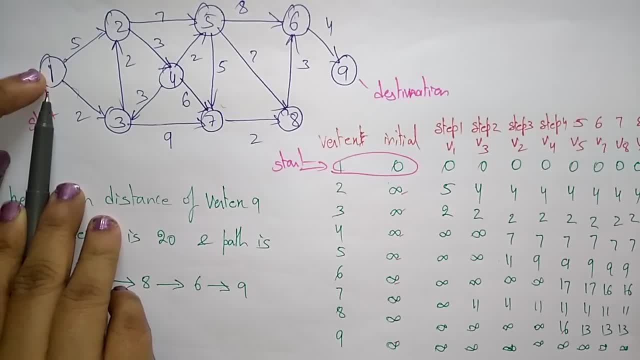 Okay, so the axis is 9 from vertex V1.. So what will be the minimum distance? so we have to be calculated by checking each vertex. Okayso, this is all comes with the vertex. 1 to 9 is the vertex. 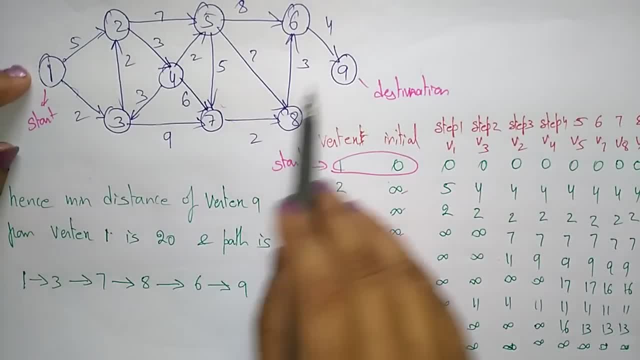 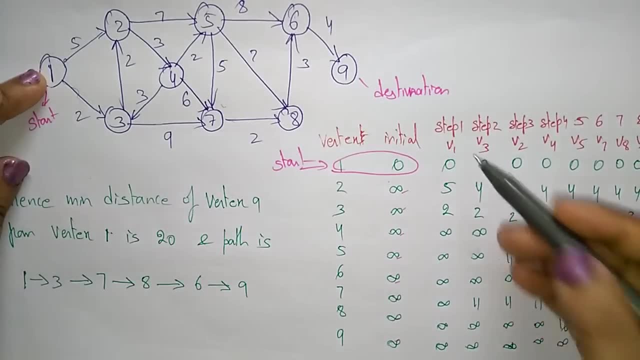 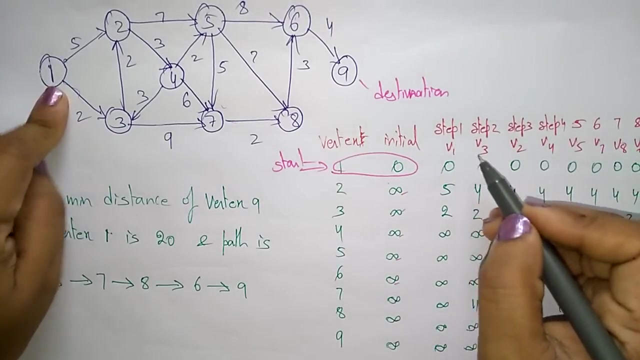 so here we have to find the minimum distance of vertex nine from vertex one. so what will be the minimum distance? so we have to be calculated by checking the each vertex. okay, so this is all. comes for the vertex one to nine is the vertex. so step one from vertex v1. so starting it is: 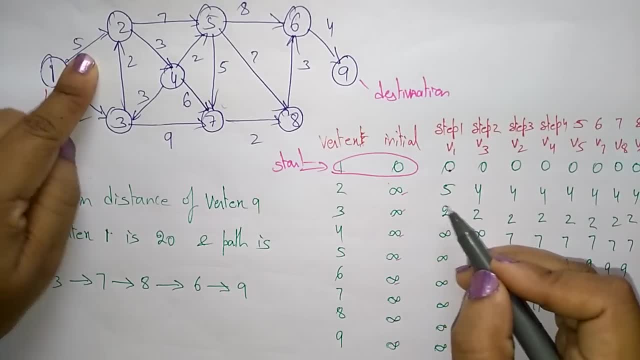 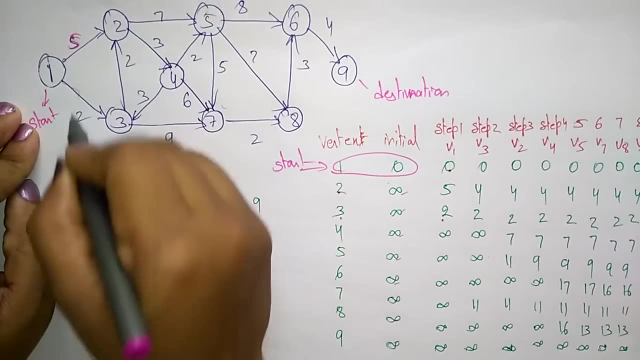 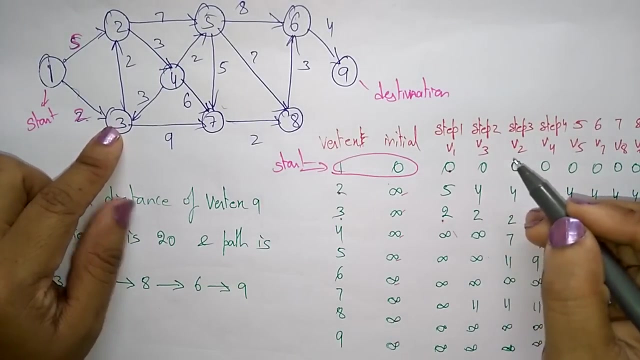 initially it is zero, marked as a zero. so the edge it has taken the five to reach to the vertex two, to reach to the vertex three, it has the edge it has taken two. so the five, two and the remaining all mark it as infinity. now coming to the vertex v3. okay, so coming. 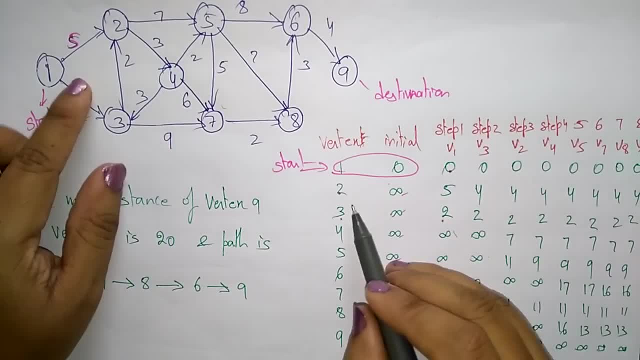 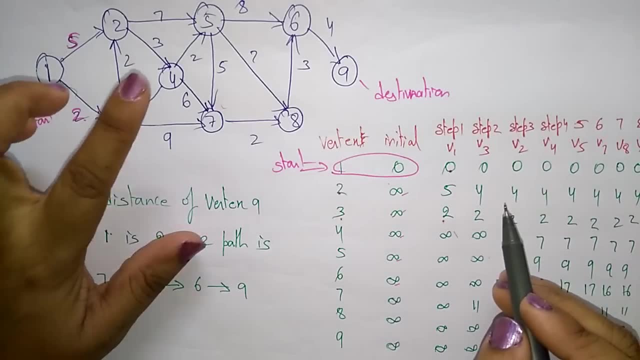 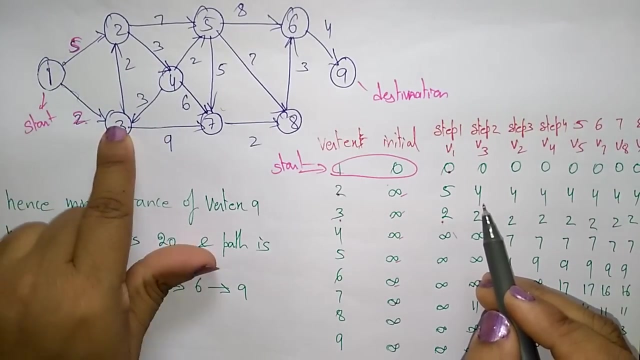 to the vertex v3. so, starting the vertex two, it has to mark it as it uh. to reach to that vertex, we have to mark it as a uh. the vertex is a four, and here the edge is coming to the three, and here, this vertex, it goes to two. so, like the 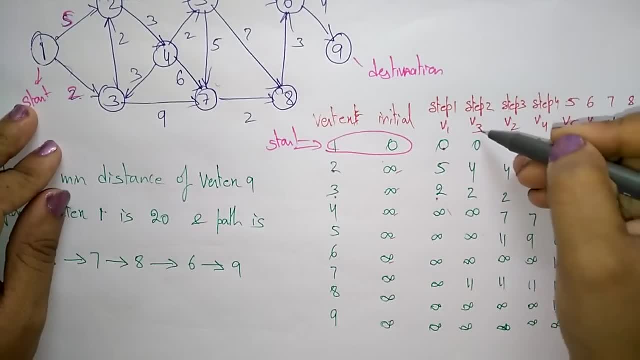 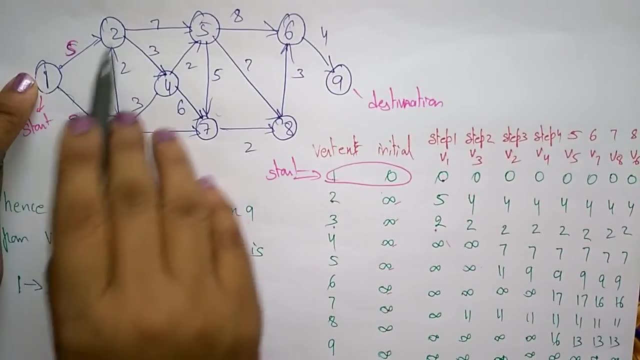 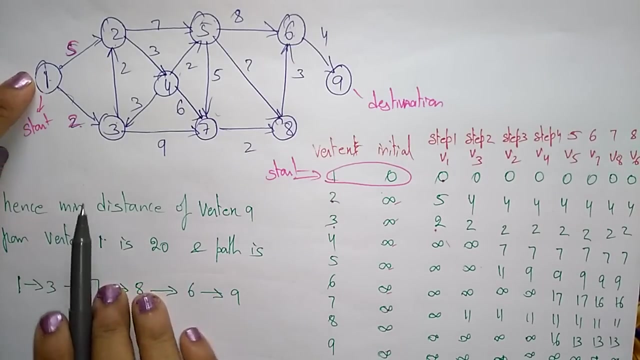 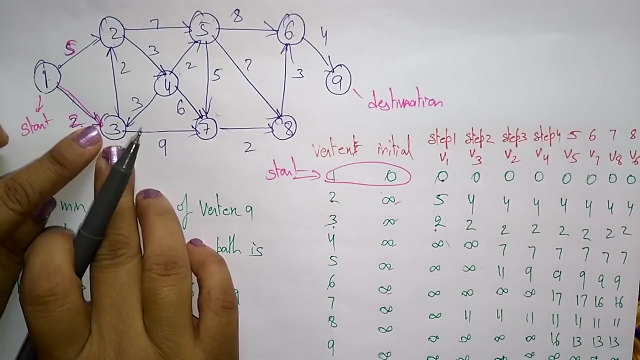 we have to be calculate. the step one, first, v1 vertex. step two: v3. step three: v2 means it's going like that, okay, so this is vertex one. this is, uh, one, two, three, four, five, six, seven, eight, totally nine vertex are there, okay? so first it goes to one, from there to v3. so this is v3, so v3, two again. 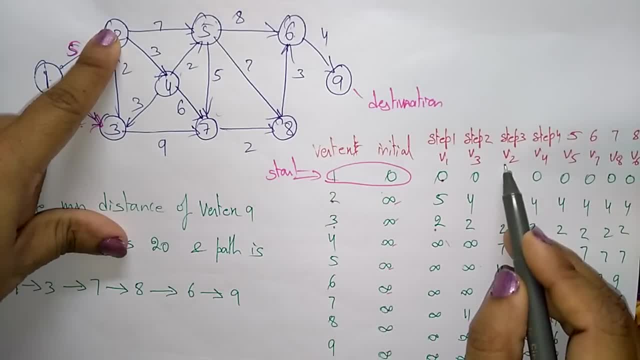 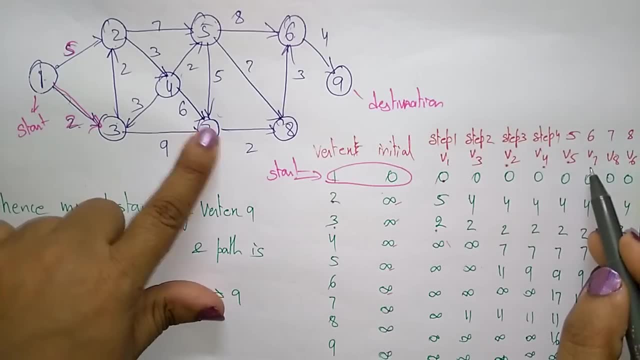 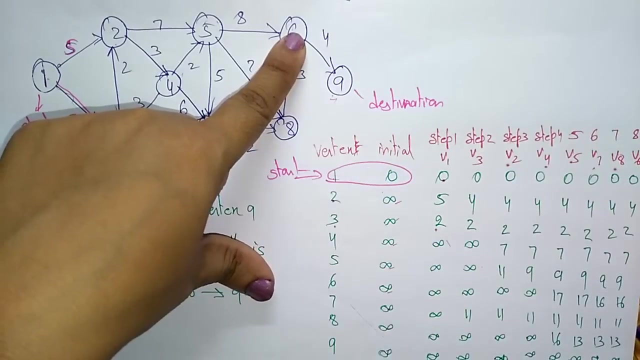 it's checking, it is going to v2, okay, so after that it going to v4. so v4 to v5, it is going to v5, v5 to v7, v7 to v8, v8 to v6, okay, finally, uh, the last one should be all, should be the infinity. 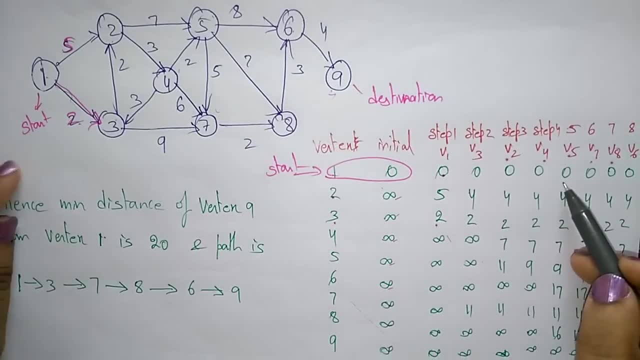 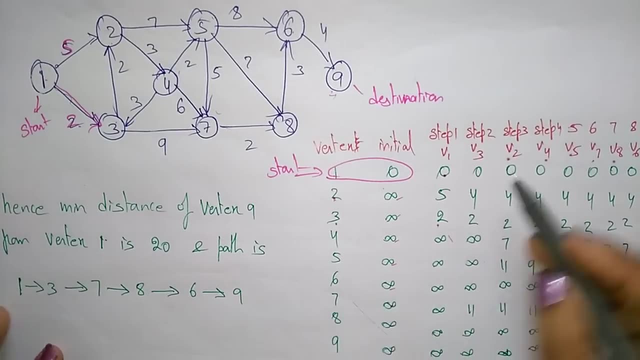 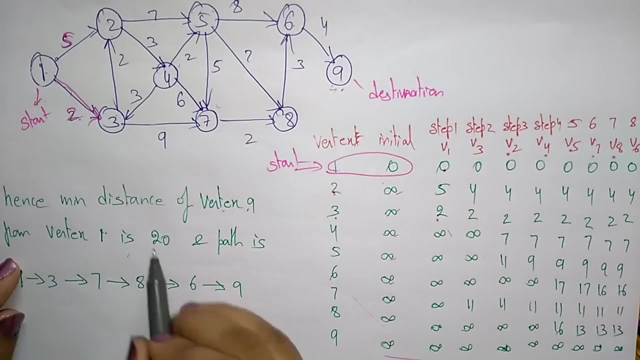 okay. so like that, it is checking each and every vertex and seeing whether that vertex contains what is the edge of that value of that vertex. so like that, we will mark the chart like this. so hence, the minimum distance of vertex nine from vertex one is 20. 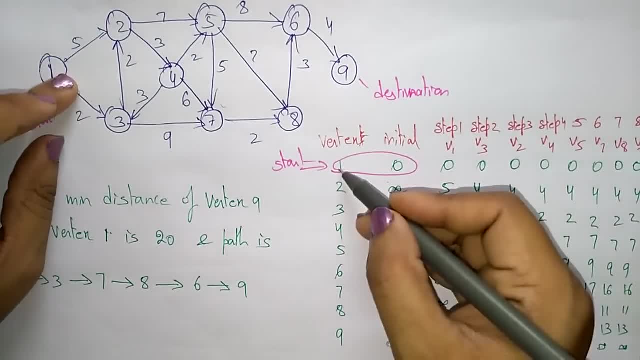 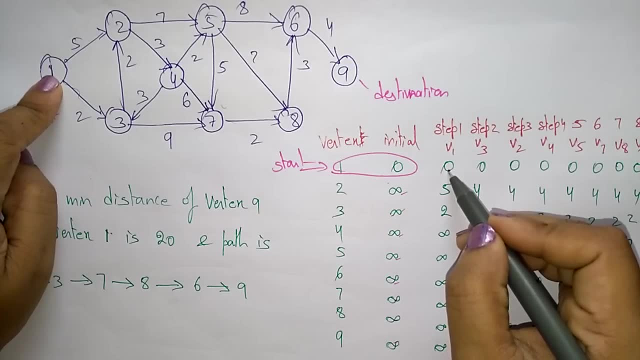 So step one from vertex V1,. so starting it is initially it is 0,, marked as a 0. So the edge, it has taken the 5, to reach to the vertex 2, to reach to the vertex 3,. 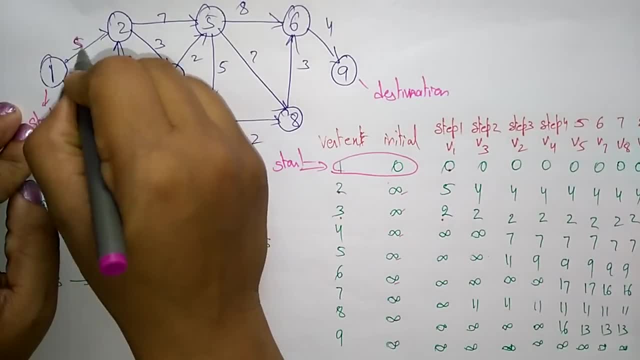 it has the edge. it has taken to so the 5,, 2. And the remaining all marked as zero. So the travelled dot 0,, 1 eh capture. And then the seek dot 0, find reached as 0,. ok, how much it has. 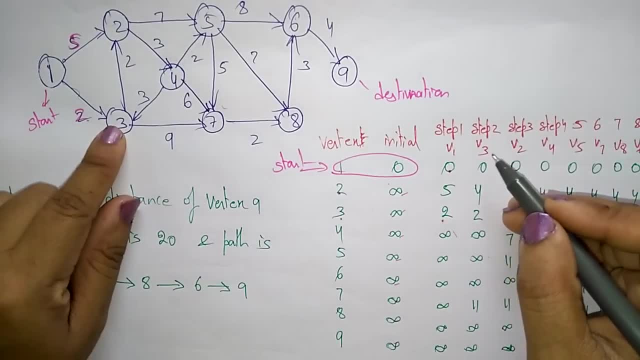 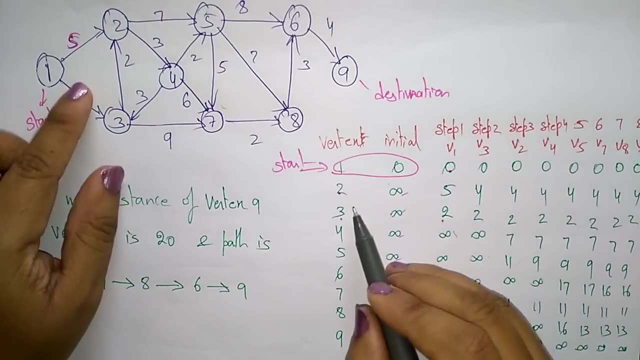 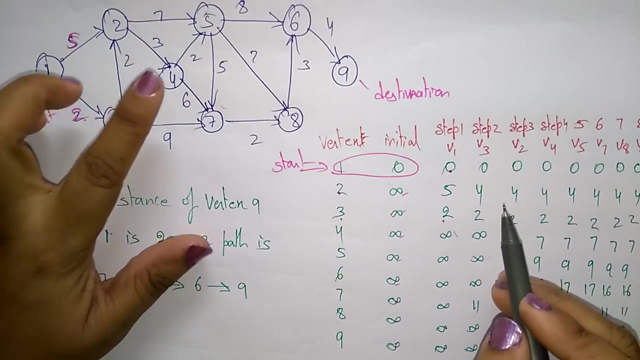 In the structure it has, And so it has to combine all at once both of them all. mark it as infinity. now coming to the vertex v3. okay, so coming to the vertex v3, so starting the vertex 2, it has to mark it as a to reach to that vertex, we have to mark it as a the vertex. 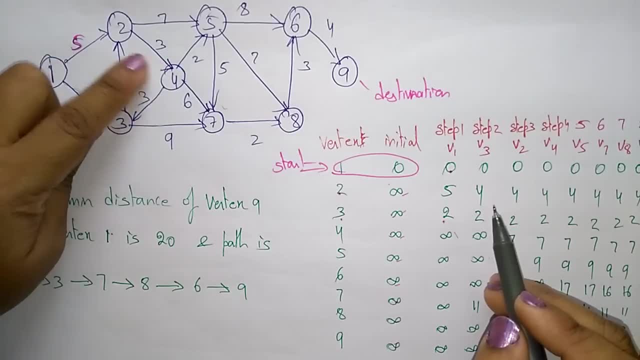 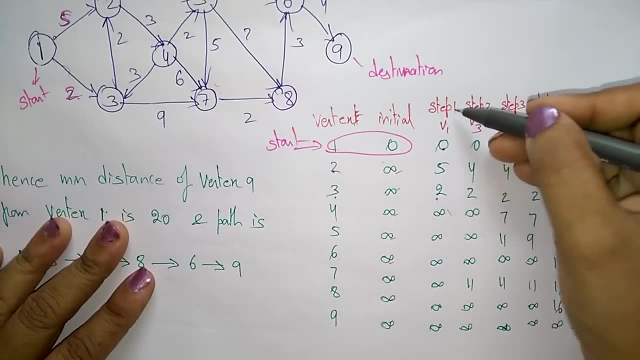 is a 4 and here the edges coming to the 3, and here, this vertex, it goes to 2. so like that we have to be calculate the step 1 first, v1 vertex. step 2, v3, step 3, v2 means it's going like that: 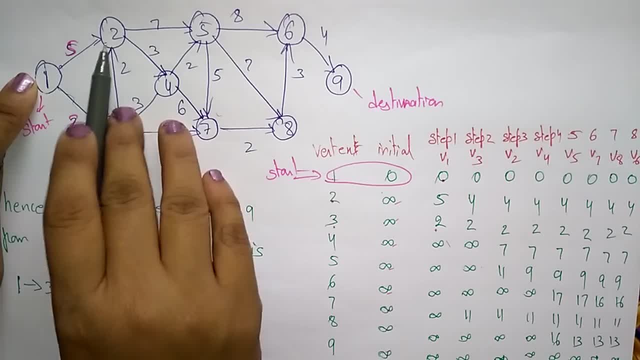 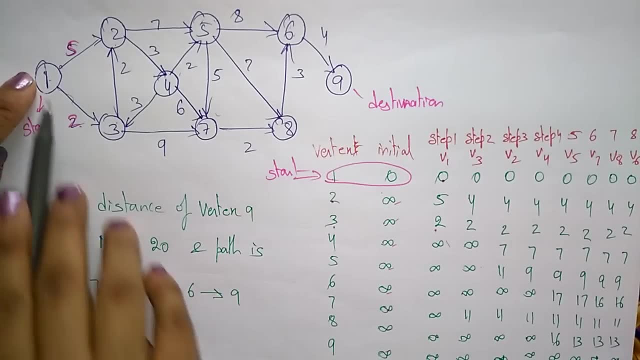 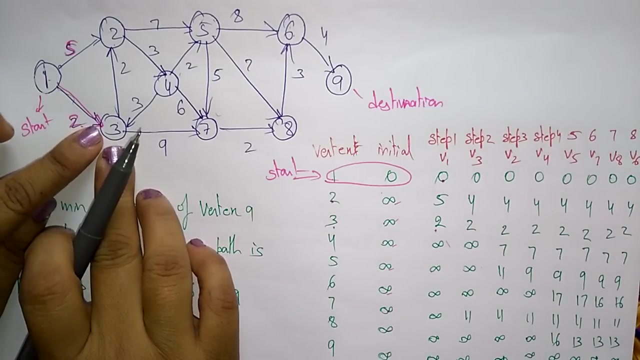 okay, so this is vertex 1. this is uh, 1, 2, 3, 4, 5, 6, 7, 8, totally 9 vertex. are there, okay? so first it goes to 1, from there to v3. so this is v3, so v3. 2- again it's shaking- it is going to v2. okay, so after the. 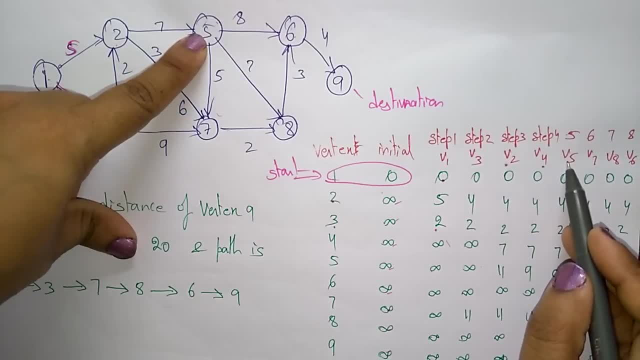 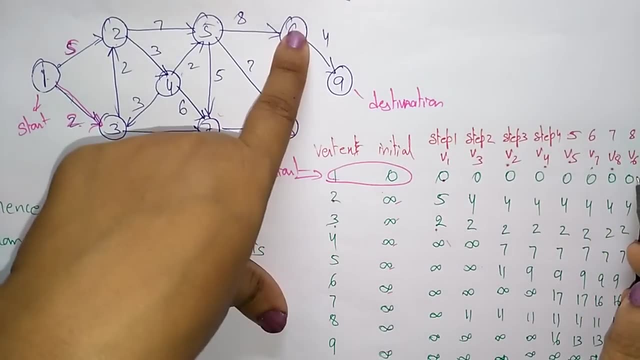 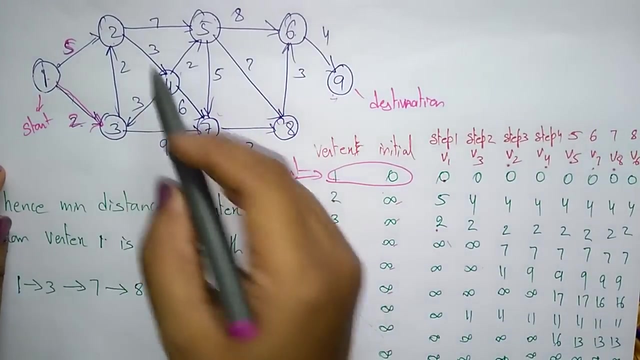 it going to v4, so v4 to v5, it is going to v5, v5 to v7, v7 to v8, v8 to v6. okay, finally, the last one should be all should be the infinity. okay, so, like that, it is checking each and every vertex and 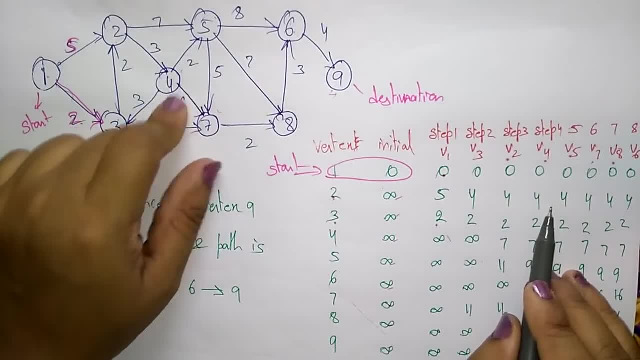 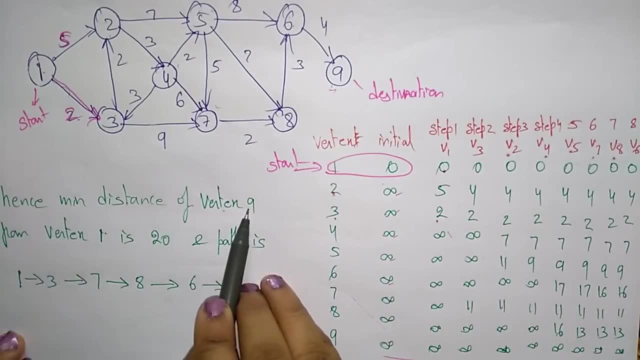 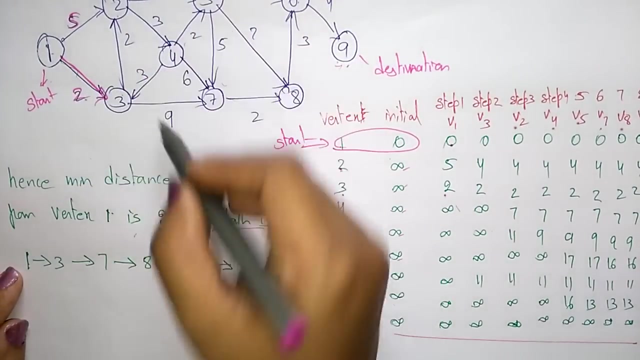 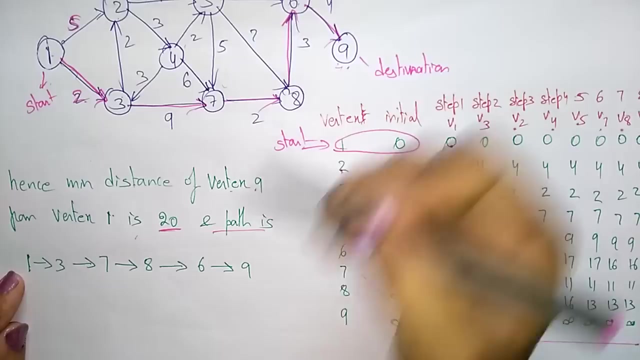 seeing whether that vertex contains. what is the edge of that value of that vertex. so, like that, we will mark the chart like this. so hence, the minimum distance of vertex 9 from vertex 1 is 20. what is the path then? 1 to 3, 3 to 7, 7 to 8, 8 to 6 and 6 to 9. so what is the total? 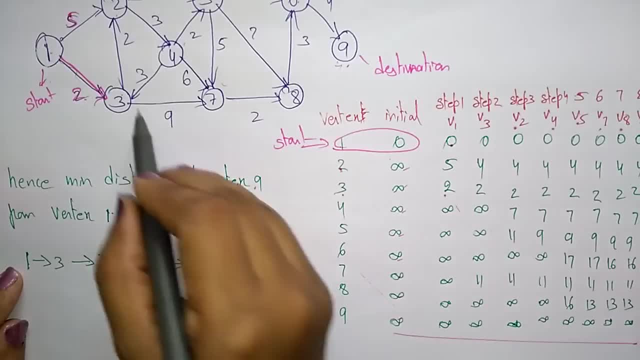 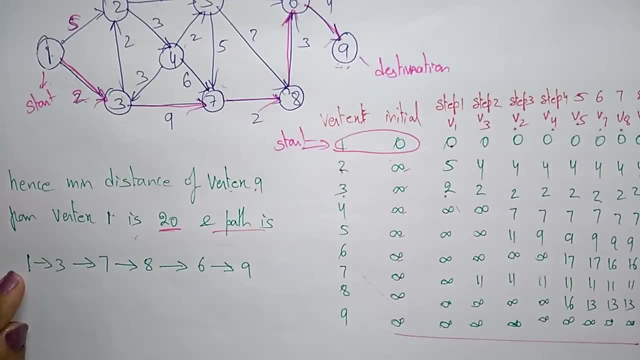 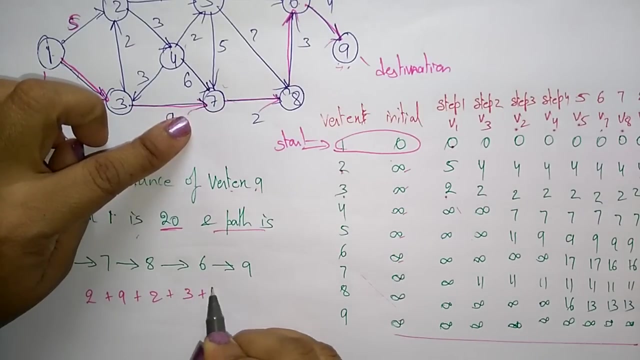 what is the path then? one, two, three, three to seven, seven to eight, eight to six and six to nine. so what is the total? two plus nine plus two plus three plus four is equal to 20, so the minimum distance from the vertex one is 20. so the minimum distance from the vertex one is 20, so the minimum